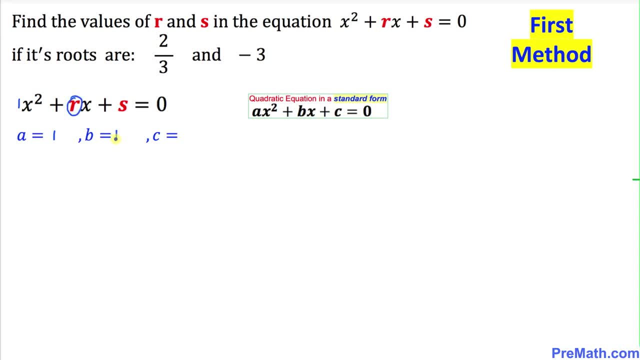 1. B value is going to be r And c value is going to be s. Now let's look at our formula. If alpha and beta are two roots of our quadratic equation, ax squared plus px plus c, equal to zero, then their sum: 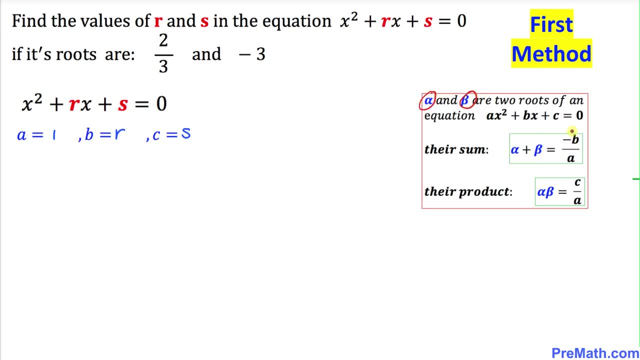 their sum of these roots is going to be minus b over a And their product is going to be c over a. And in our case this two-third is our alpha and negative three is our beta. Two roots, And here we are going to find the sum alpha plus beta. That means we're going to add these. 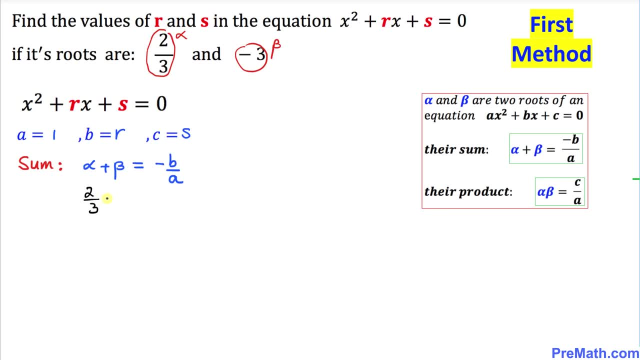 two roots, Two over three plus this beta is negative. three equal to. in our case, b equals to r, So that's going to become negative. r divided by a is one. Let's simplify this thing On the left-hand side. that's going to give us two-third positive, and negative becomes negative. three equals to. 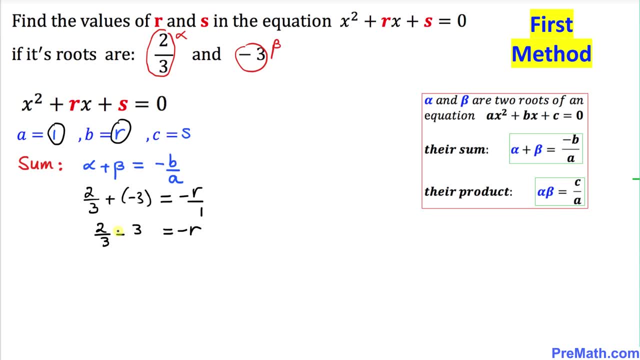 negative r. Now let's simplify the left-hand side. I can make this three as a fraction, just putting one underneath. I can just simply cross, multiply, crisscross. All right, Let me show you how we're going to do it. 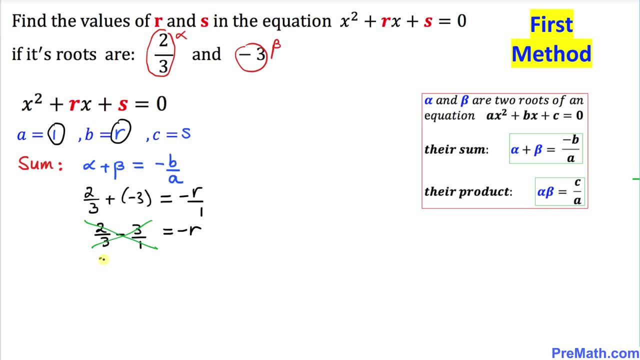 Really simple: Two times one- This way is going to be two minus whatever this sign is. And then three times three is nine, divided by whatever our denominators are, three and one. We are going to multiply them out. That's going to give us: three times one is three And that is going 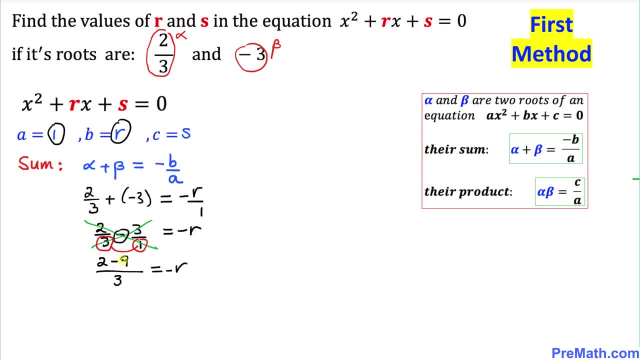 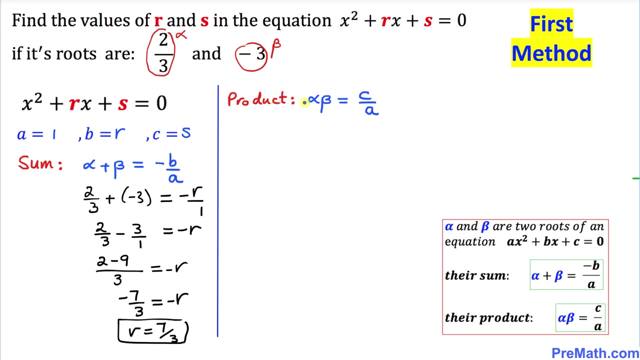 to be equal to negative r. So this, on the top, is going to be negative. seven over three equal to negative r. So negative and negative cancels out. So our r value is going to be seven-third. In this next step we are going to find the product of these two roots: alpha times, beta. 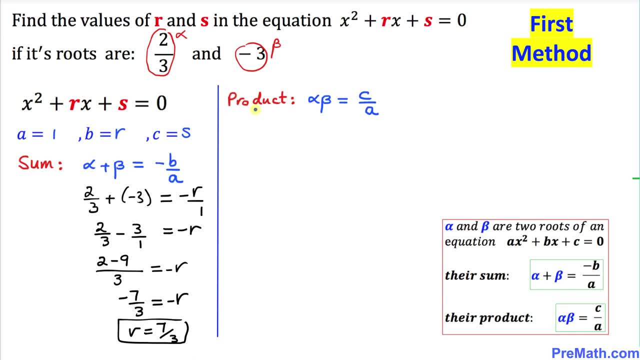 equal to c. In our case, alpha is two-third- Just write it down- And our beta is negative. three equals to: in our case c is s. Just let's put down: s divided by a is one, And, as we can see that this 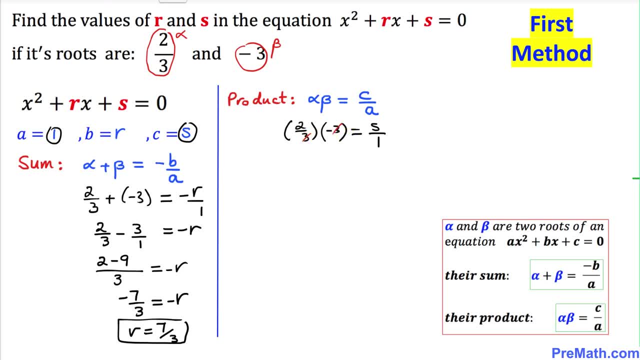 three and this three, this is gone. So we ended up on the left-hand side. This side is gonna be on the right-hand side and our top is gonna be safety and our bottom is gonna be safety and he's gonna be safety. 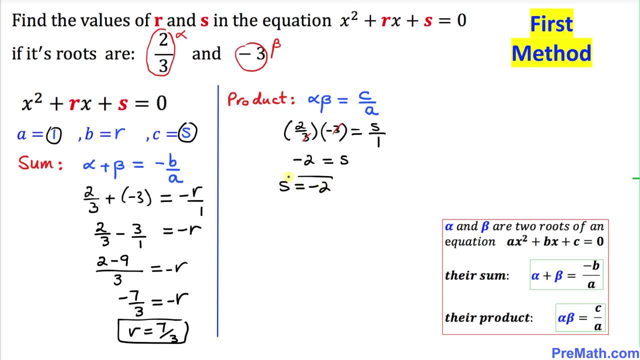 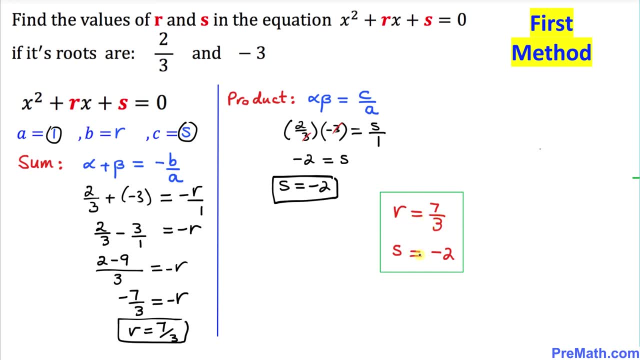 So remember that both sides have them And we're gonna write down our ladım- okay, Because w is on our top. We're gonna know what's the value when we put down w equal to seven-third and w is not a value of five. We can belong this modprocess, peoples. 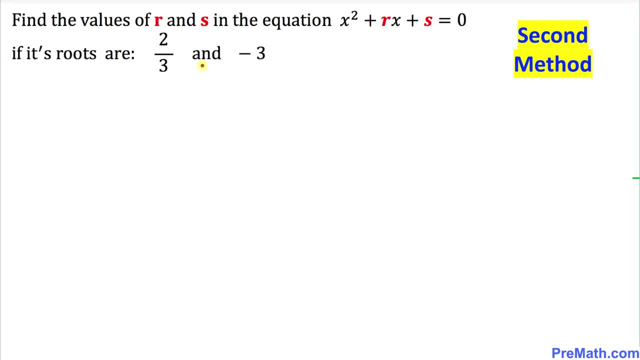 we're gonna know what the value is when we put down. let me show you. We're gonna say that we're gonna be using one of these two groups. Let me just write down one of these, And we are going to use this really simple formula: x minus the first root, which is this one: 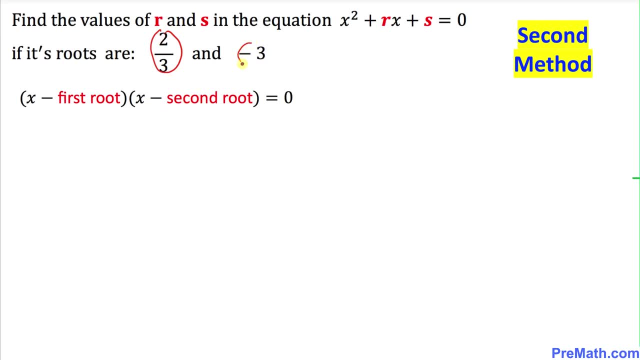 and times: x minus the second root, which is negative, 3 equal to 0.. Let's go ahead and fill in the blanks. So x minus this first root is 2. 3rd- I'm going to just write down 2, 3rd times. 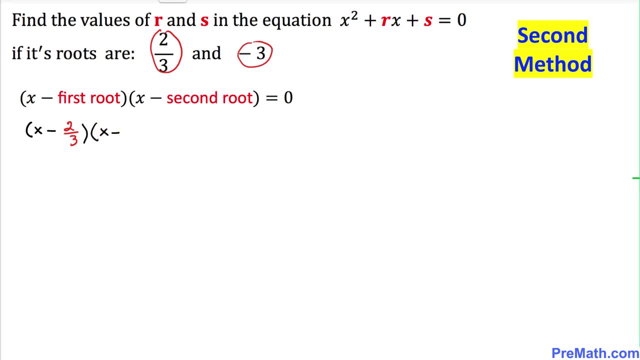 and then x minus the second root is negative 3 and parentheses close- equal to 0.. And now let's focus on this very first factor: x minus 2- 3rd. I just copy it down over here: x minus 2- 3rd equal. 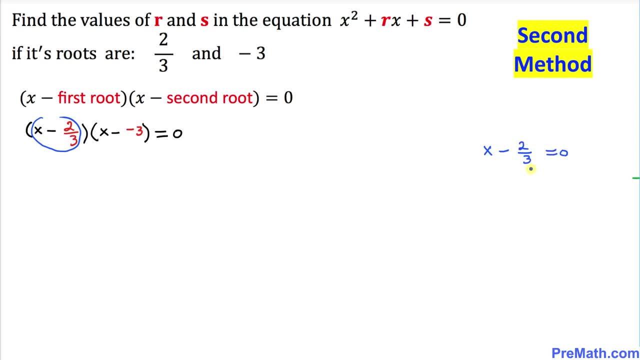 to 0.. Let me show you an easy way to remove this fraction. Let's focus on this denominator 3, and then x minus the second root is negative 3 and parentheses close- equal to 0. And now let's simply drag it and put it in the front. That's all we have to do, So that could be written as: 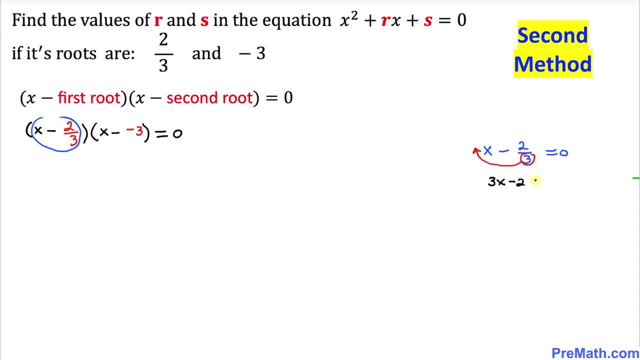 3x minus 2 equal to 0. So thus we can write this first vector nicely as 3x minus 2 times. See, we have a two negative signs. They are multiplying. That is going to give us negative times. negative is positive, So we are going to write this first vector nicely as 3x minus 2 times negative times. 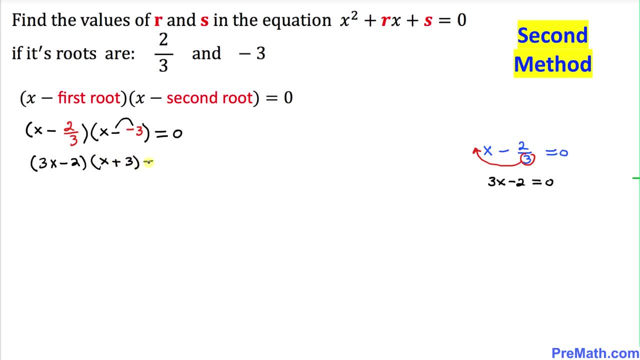 positive. So x plus 3 equal to 0.. And now we are going to use this FOIL method. Let's see how we're going to do: is 3x times x and then 3x times 3.. Let's go ahead and do this thing. So 3x times x. 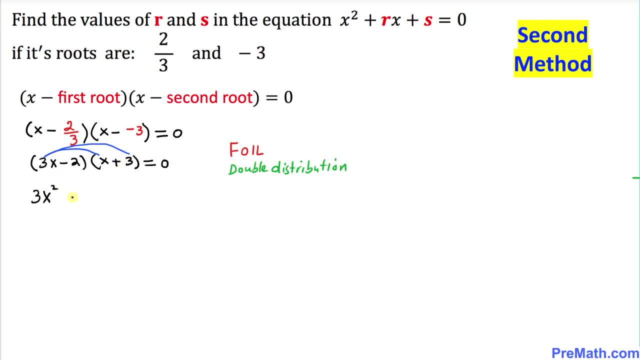 is going to give us 3x squared. 3x times 3 is going to be plus 9x. And now we're going to distribute once again. No wonder we call it double distribution: Negative 2 times x and negative 2 times 3.. So that's going. 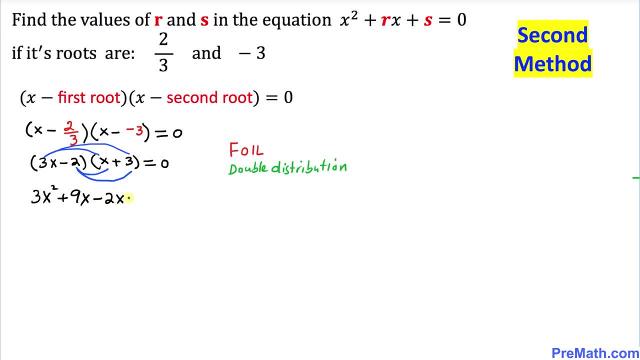 to give us negative 2x, negative 6, equal to 0.. Now let's go ahead and combine the like terms So this could be written as: 3x squared, 9x minus 2x is going to be a positive 7x minus 6.. 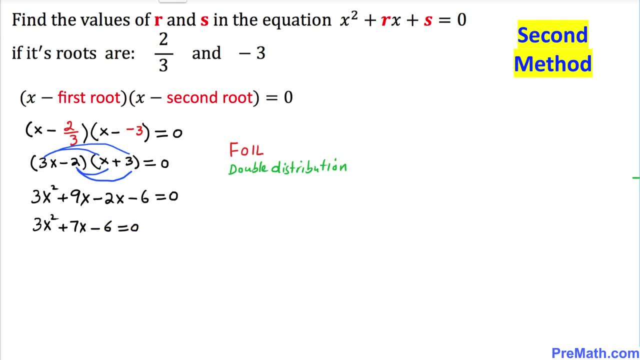 Yeah, that's actually our negative Racing Japanese. So we wrote negative x squared in there and negative 6.. So we know negative x should be zero, as we except negative 4 minus 1.. 111 subject and minusолетous and negative minus 7 eltones equal to 0.. And we want to make sure that our leading coefficient is one. So I, Senator of 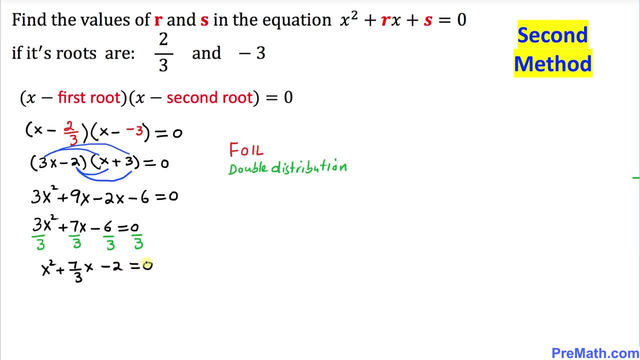 the board each and every term. So this could be written as simply a square plus 7 over 3 x minus 2, equal to 0.. And here is our North Texas test. So we are going to do 3x times 3, 7 minus 3 times negative, 9 distributed Now. 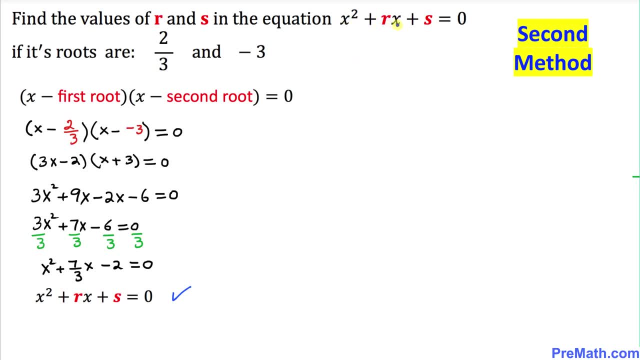 given quadratic equation: x square plus rx plus s, equal to 0, and we are going to compare their coefficient and, as we can see, that r is going to be 7, third and s is going to be negative 2.. So r turns out to be 7 over 3 and s is negative 2.. Thus our r and s values turn out to be a 7.